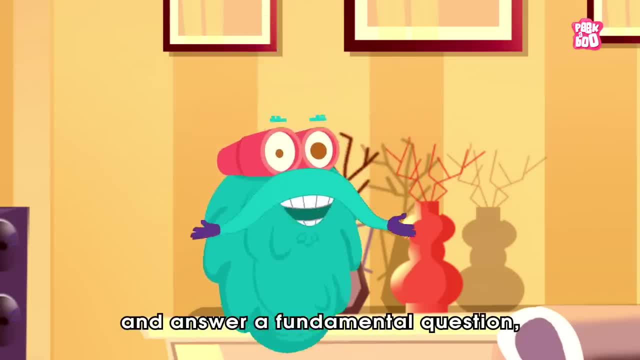 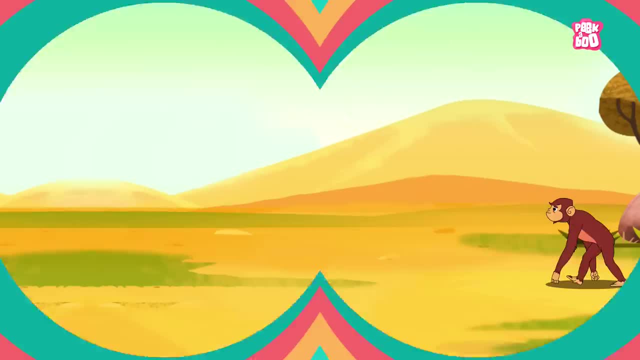 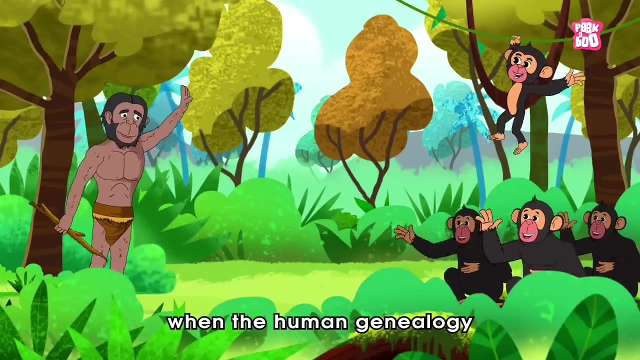 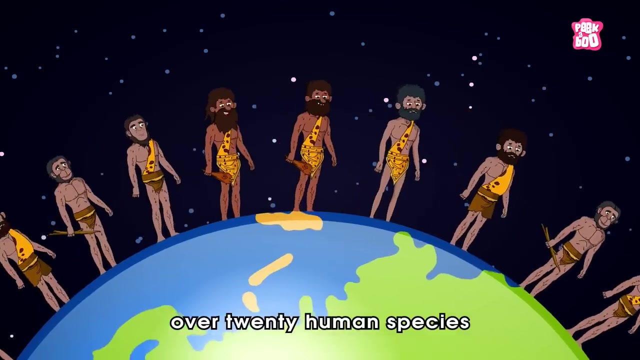 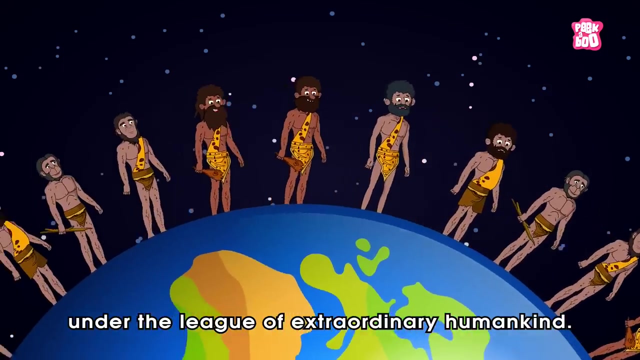 Yes, you the humans, and answer a fundamental question: Where did humans come from? Zoom in: The human evolution started nearly 7 million years ago, when the human genealogy separated from the chimpanzees and, as the time passed by, over 20 human species or hominin originated under the lead of extraordinary humankind. 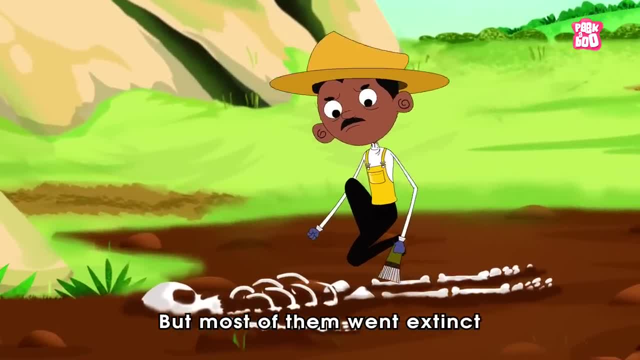 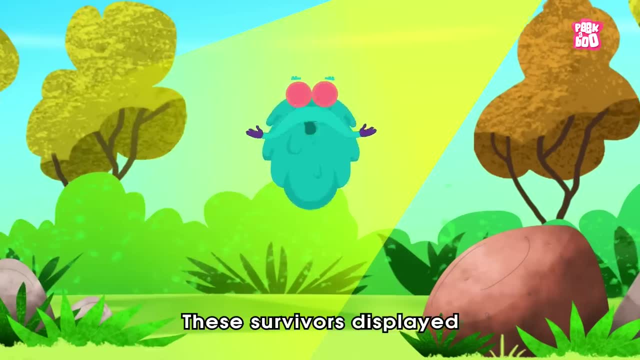 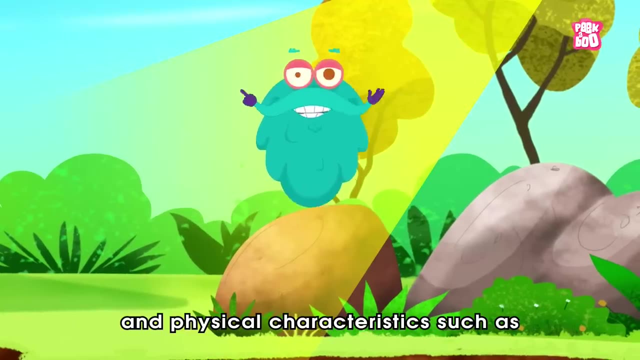 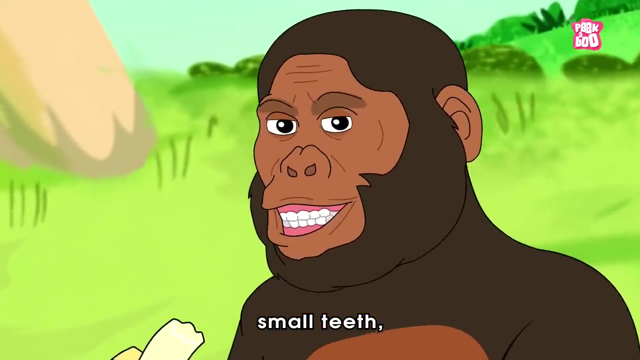 But most of them went extinct, while those who survived might have been ancestors of modern humans. These survivors displayed various human-like psychological, behavioral and physical characteristics, such as large brains, the ability to walk on two legs, small teeth and the skill to carve and use tools and weapons. 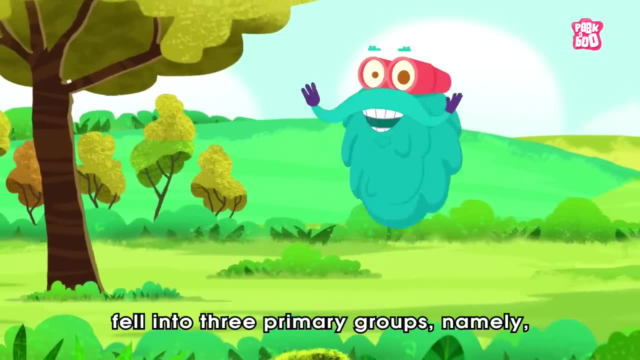 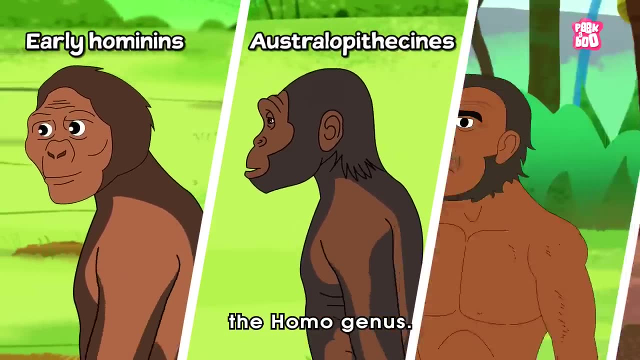 These smart creatures fell into three primary groups, namely early hominins, australopithecines and the Homo genus. The early hominins are believed to exist between the early and the late Homo genus. The early hominins are believed to exist between the early and the late Homo genus. 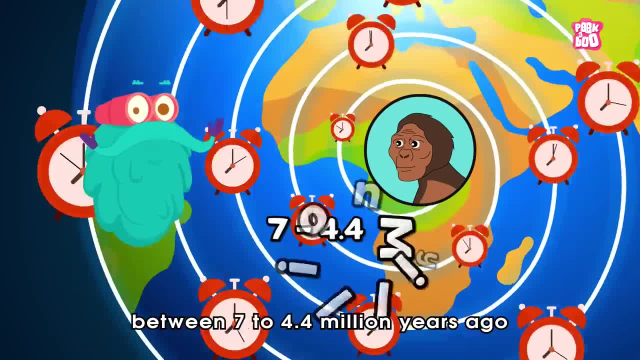 The early hominins are believed to exist between the early and the late Homo genus. The early hominins are believed to exist between 7 to 4.4 million years ago in the great African continent. The early hominins are believed to exist between the early and the late Homo genus. 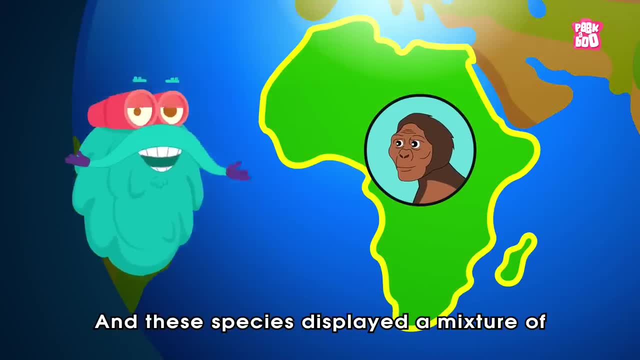 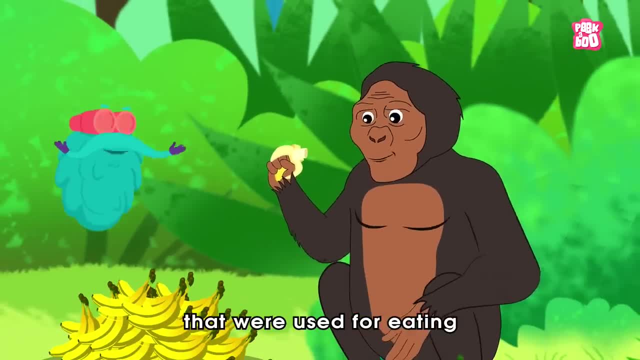 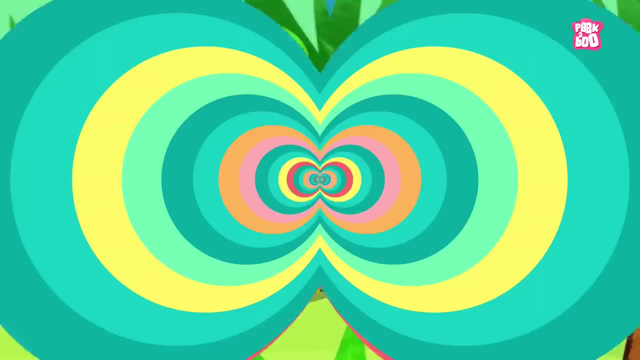 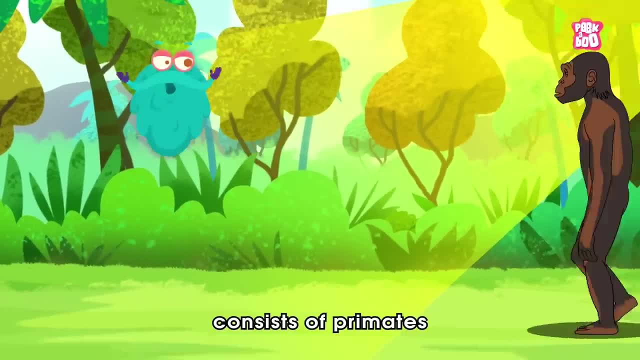 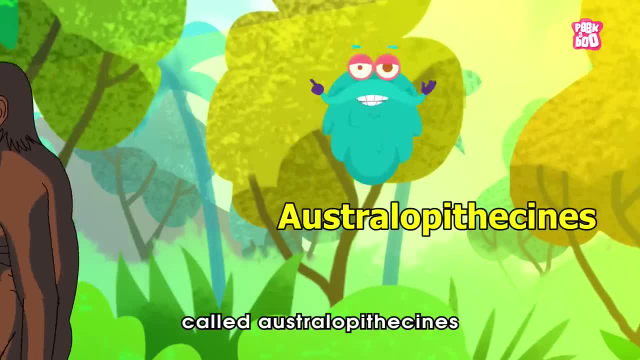 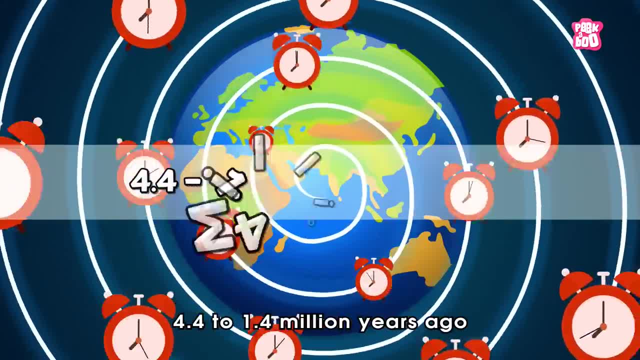 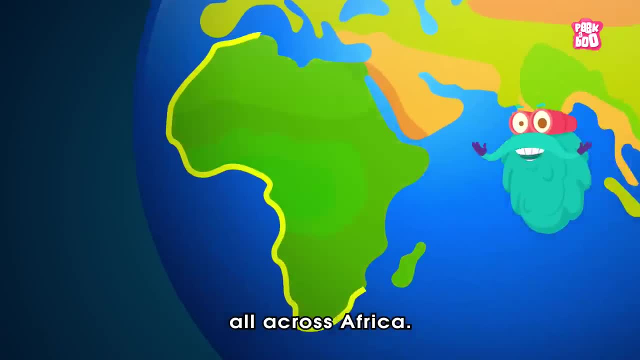 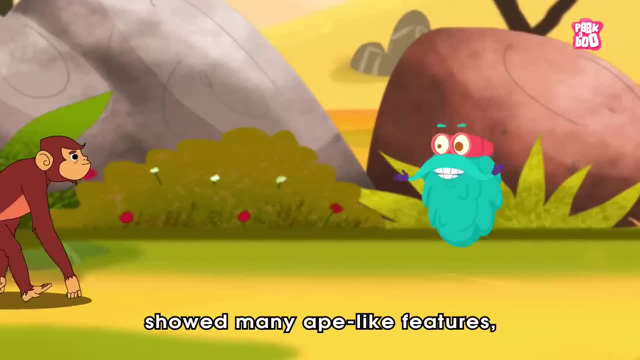 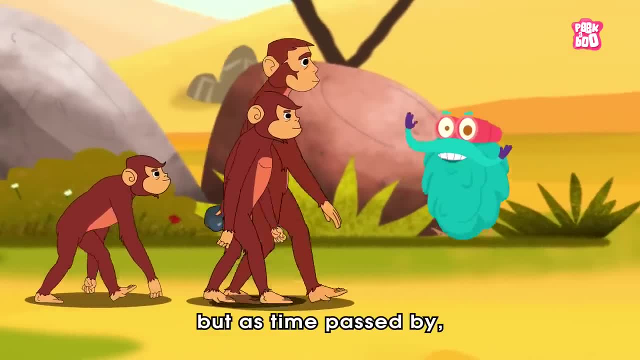 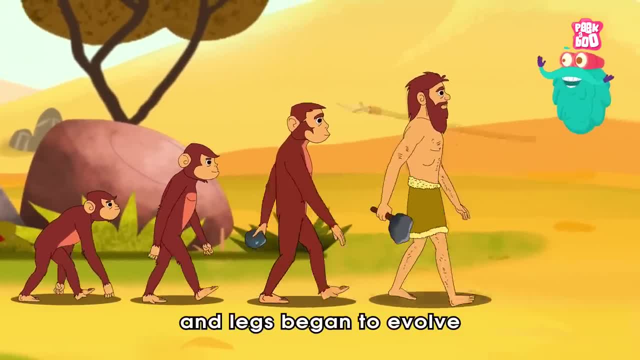 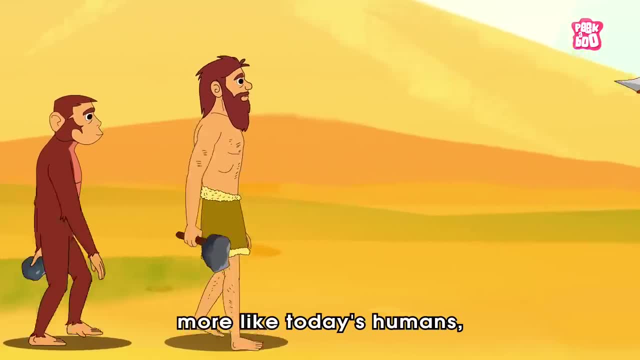 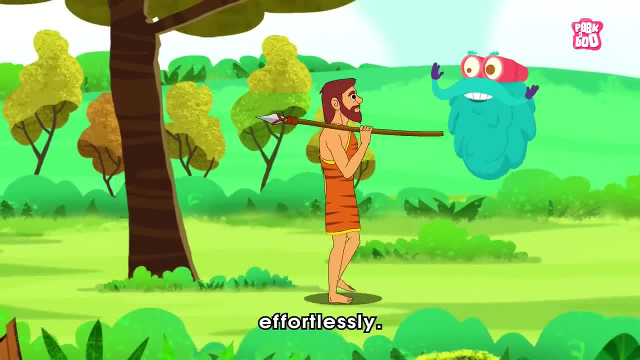 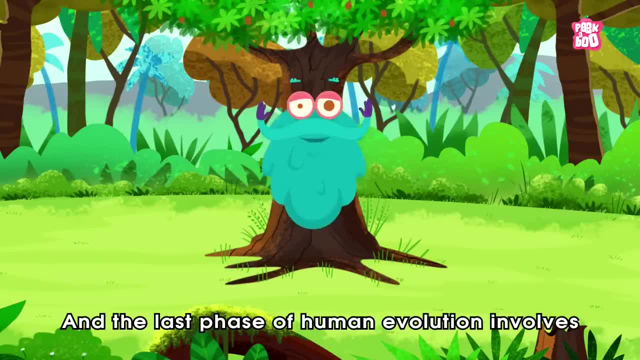 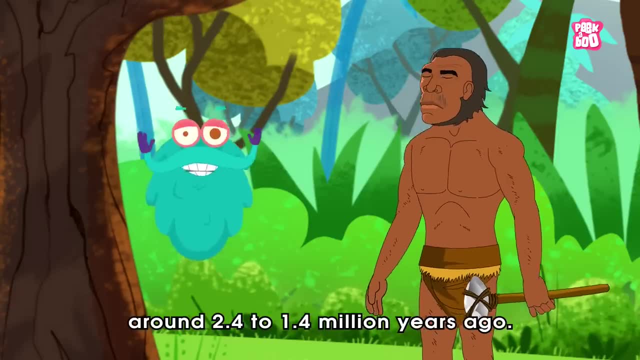 And these species displayed a mixture of ape and human characteristics, like small teeth that were used for eating instead of hunting and fighting. The last phase of human evolution involves the homogenous family that are believed to come into existence around 2.4 to 1.4 million years ago. 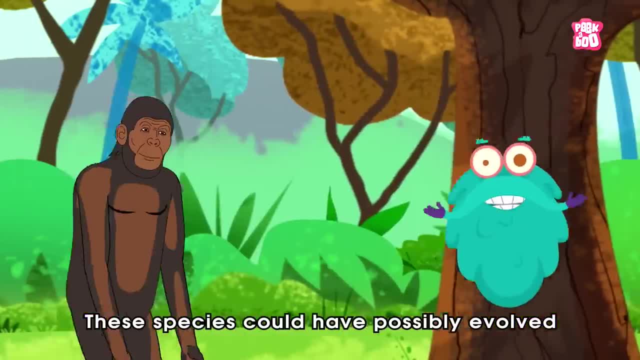 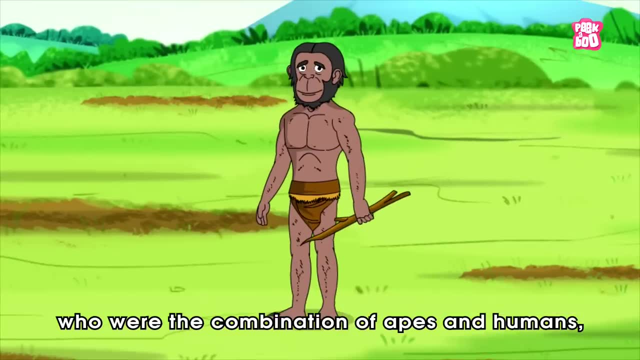 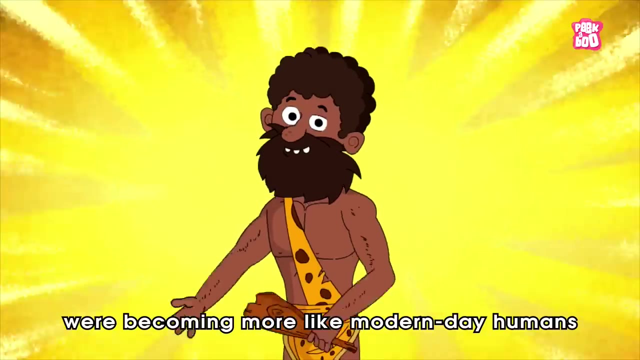 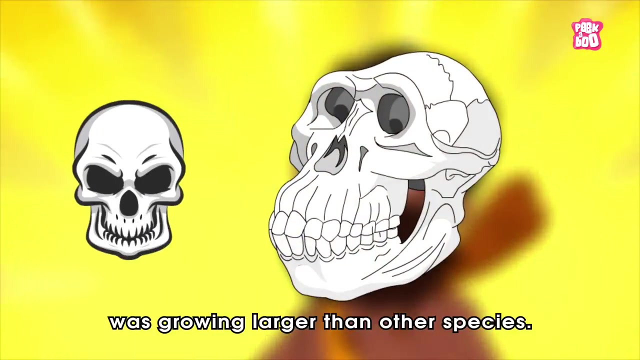 These species could have possibly evolved from the Australopithecine lineage, But unlike Australopithecines, who were the combination of apes and humans, the Homo species were becoming more like modern-day humans, as their inner skull size was growing larger than other species. 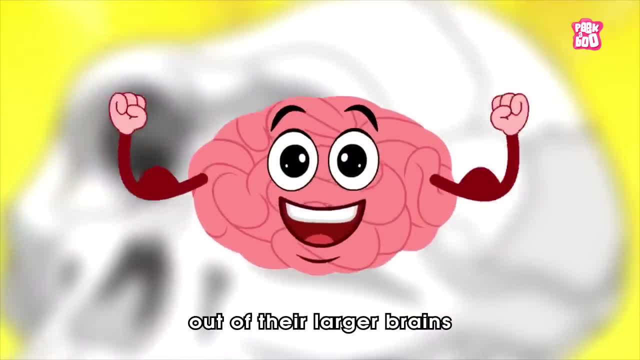 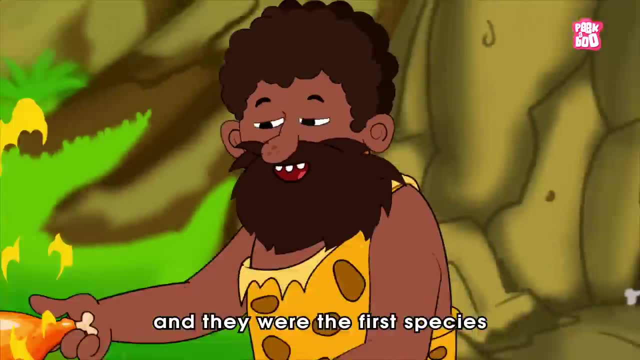 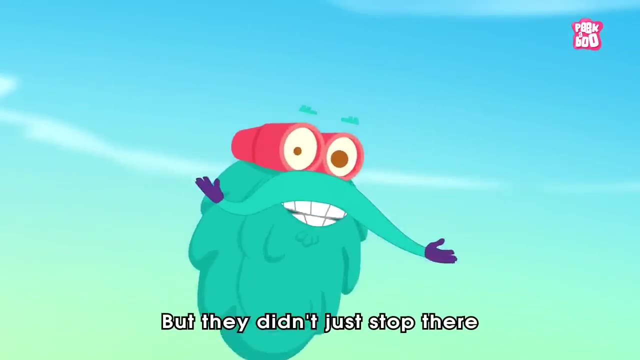 And they made the most out of their larger brains by developing hunting techniques with the help of better tools, And they were the first species to utilize the burning capacity of fire. But they didn't just stop there, These improvements in physical, mental and behavioral characteristics. 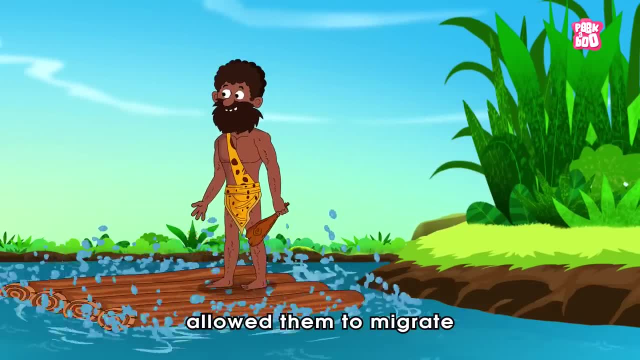 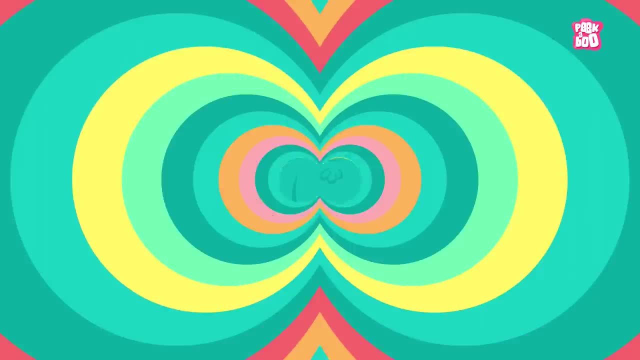 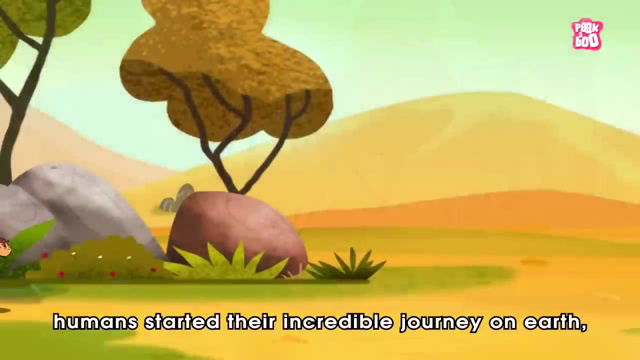 combined with advanced technologies, allowed them to migrate out of Africa and explore the other parts of the world. So, my friends, although more than 20 species of humans started their incredible journey on Earth, in the end only one, the Homo sapiens.